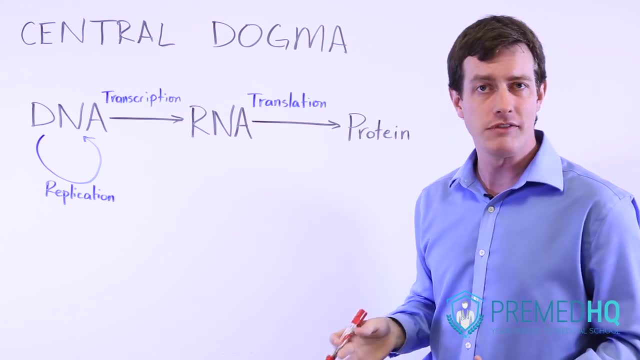 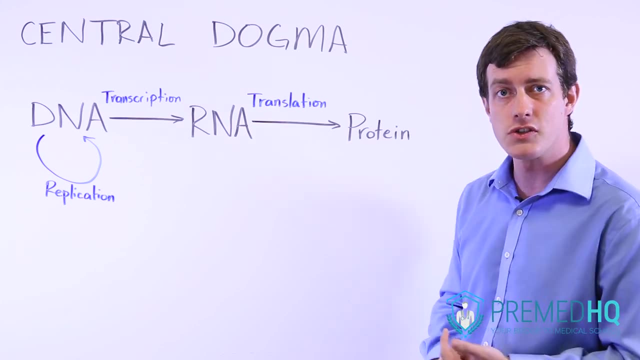 that participate in all of these steps and they can be very confusing. You have RNA polymerases and DNA polymerases, You have promoters and transcription factors, You have tRNA and mRNA, And the best way to organize all that information in your mind is to think. 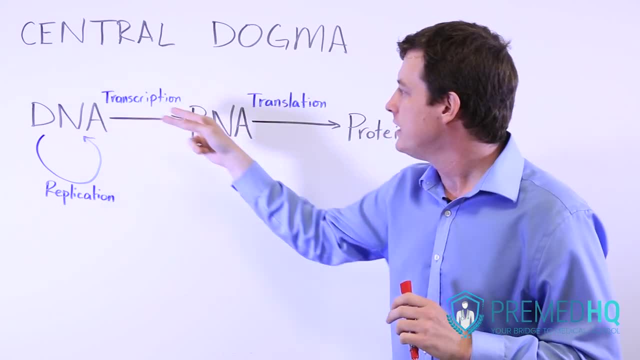 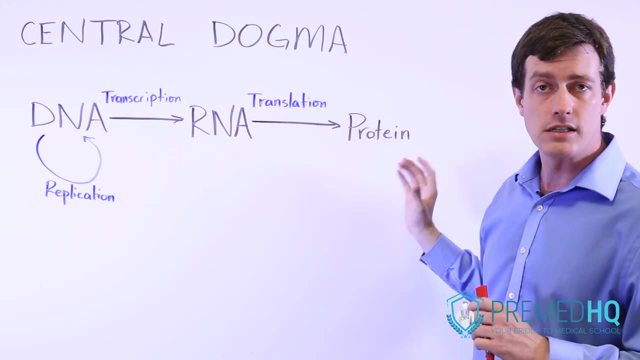 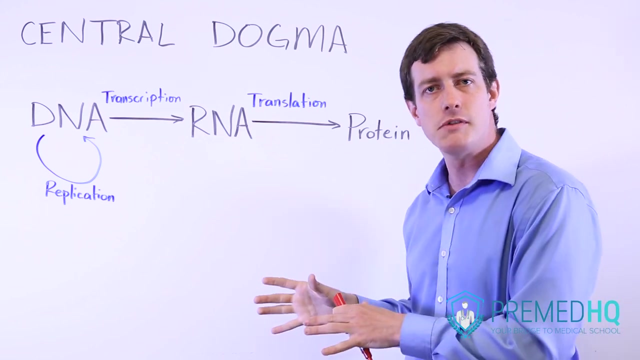 of everything in terms of the central dogma and the steps that go on as this process advances to this and as the RNA is then translated into protein. But notice here that we've also added replication, DNA replication- because oftentimes students will confuse that with, for example. 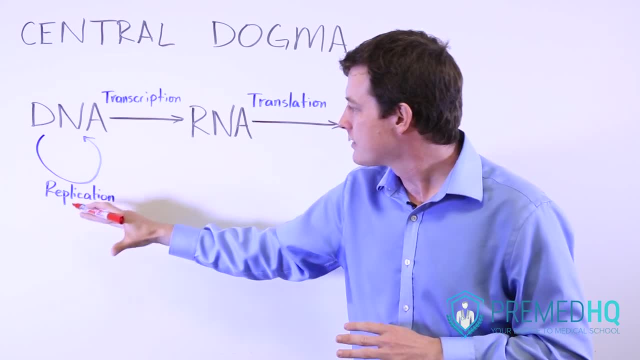 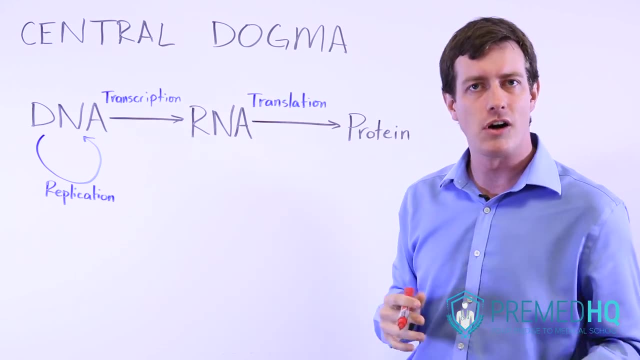 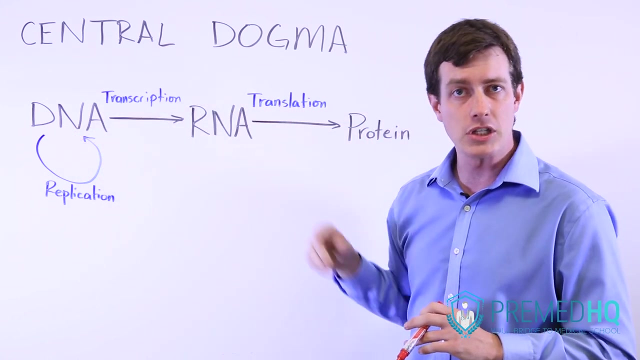 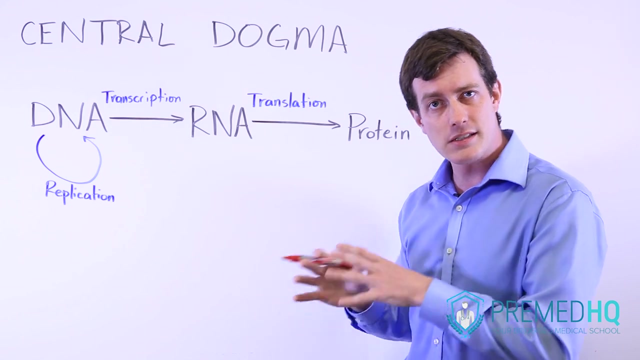 transcription, And it's important to recognize that this is also a separate component that involves its own enzymes and its own protein factors That also participate. And so, in general, the transition from DNA to RNA, it's called transcription And it involves an RNA polymerase. It involves some transcription factors. Then you have to splice. 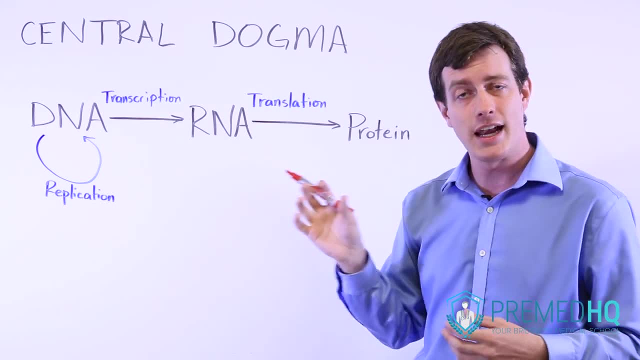 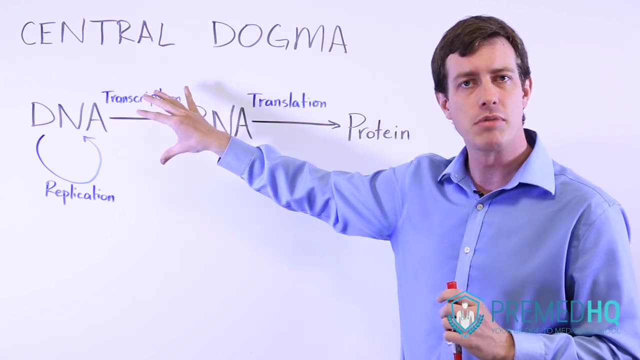 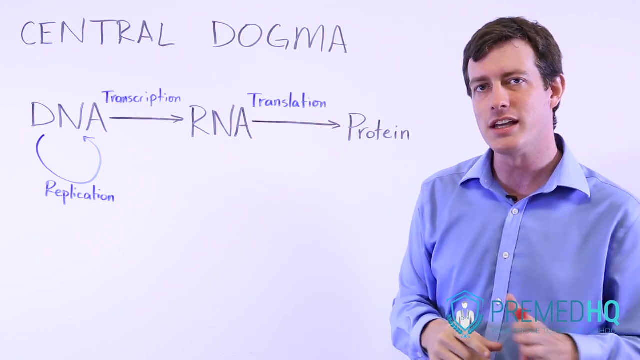 the primary transcript and then process it by adding a cap and a tail to enable it to then reach the cytoplasm. So transcription has many different components of its own. And then, when the RNA goes out to the cytoplasm, that's when the translation process begins And that's when your processed mRNA is then. 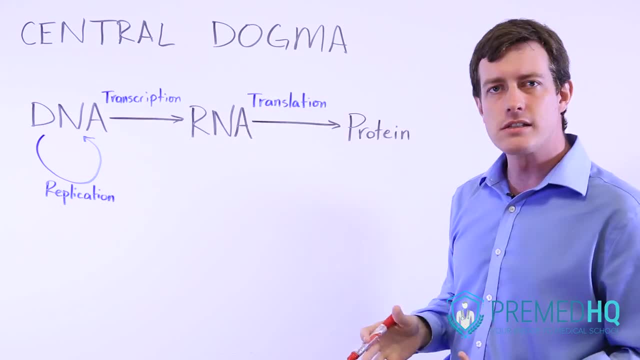 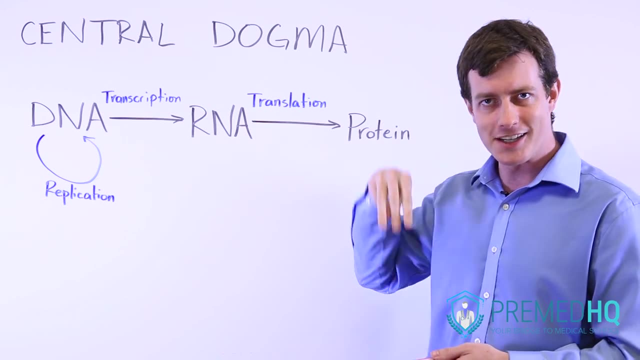 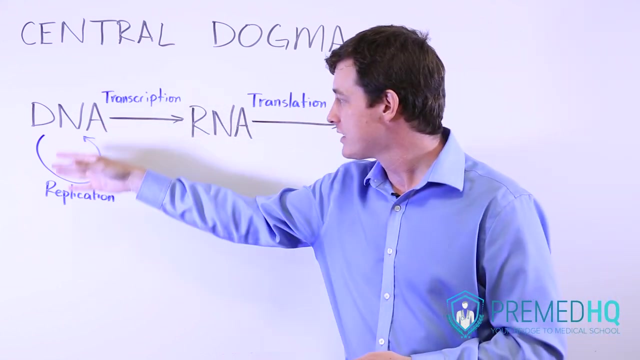 translated into proteins in a system that involves ATP usage and some tRNAs that enable you to link your mRNA codons with the proteins that are being built from amino acids. And then replication has its own set of factors. It has helicases that unwind. It has single strand binding proteins. 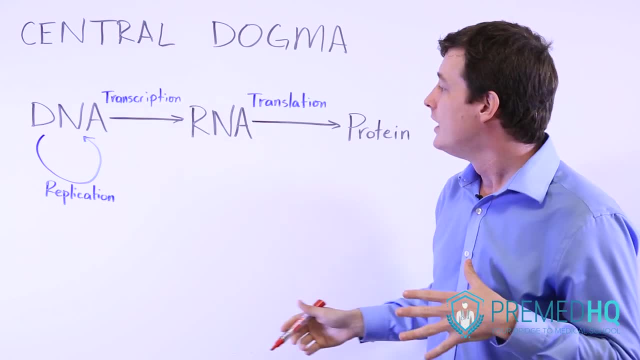 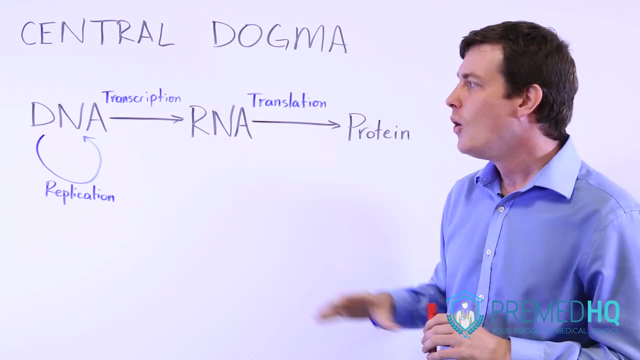 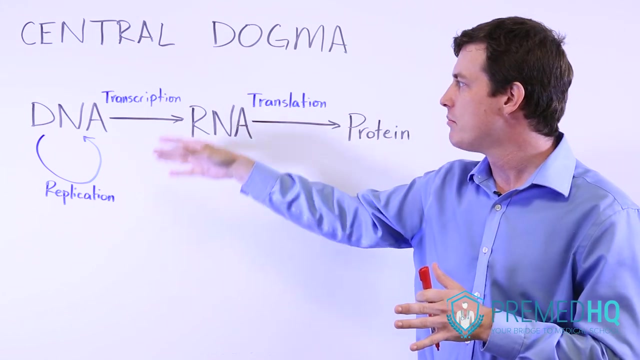 that help stabilize the two parent template strands, And it involves DNA polymerases, primers and different components like that, And so while you're working through all of these, it's important to keep the central dogma in mind, And we'll have videos going through each step in. 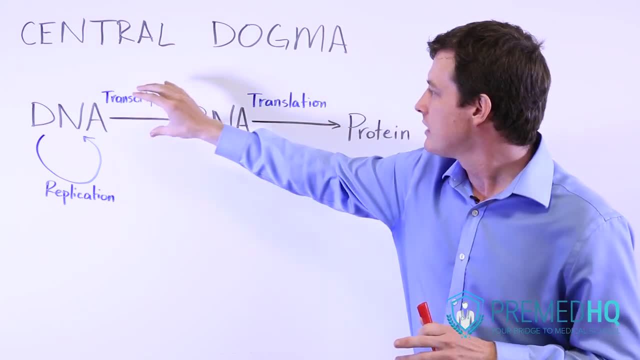 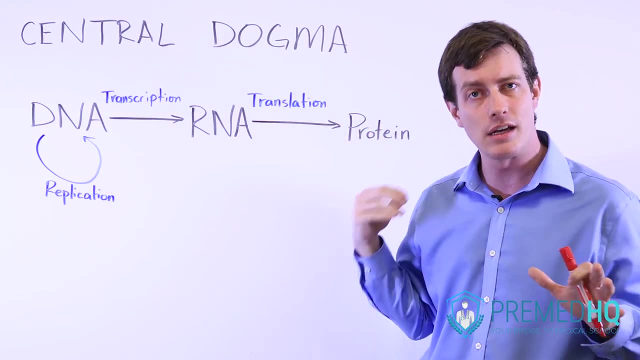 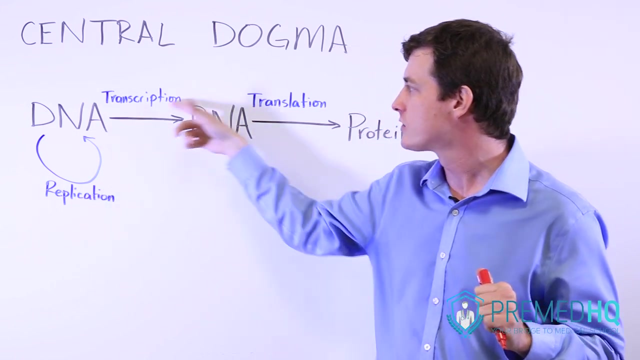 this process And if you then are able to isolate these three different things as three separate processes, then you'll have a much bigger picture understanding and it will help you answer questions where they might try to trick you into using a DNA replication enzyme to answer a.